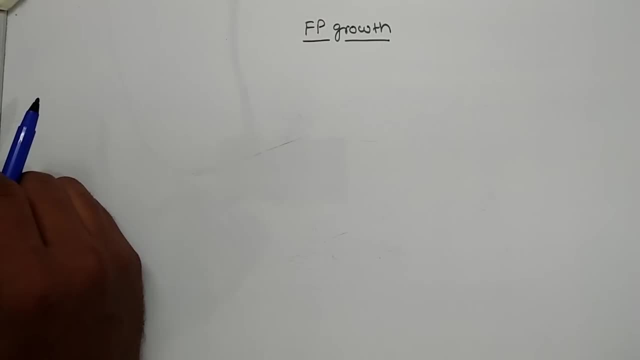 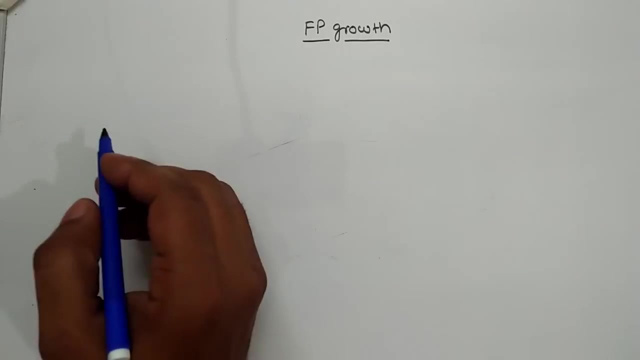 Hello guys, we continue our lectures on association analysis. In this lecture we will learn about second algorithm of association analysis, that is, frequent pattern growth algorithm. Previously we have studied a priori algorithm. There are some of the drawbacks of a priori algorithm and to remove those drawbacks we have to study the FP growth algorithm, The main drawback. 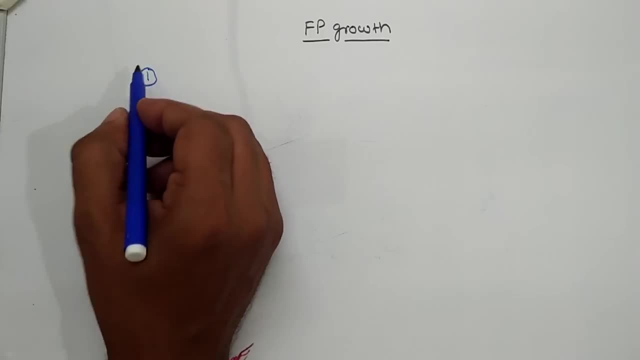 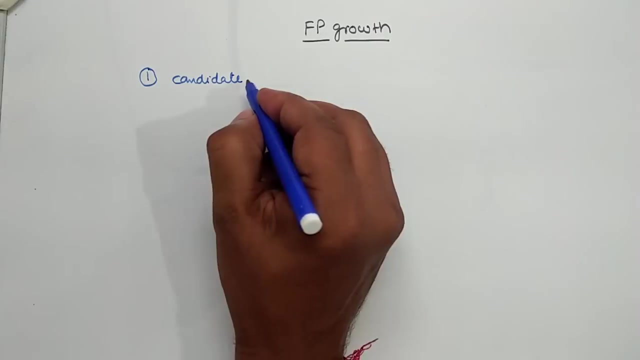 of a priori algorithms are. first is at each step, we have to calculate the candidate patterns, We have to search for the, we have to find out the combinations of frequent pattern in order to find out the candidate sets of the pattern, And it is if the frequent items are. 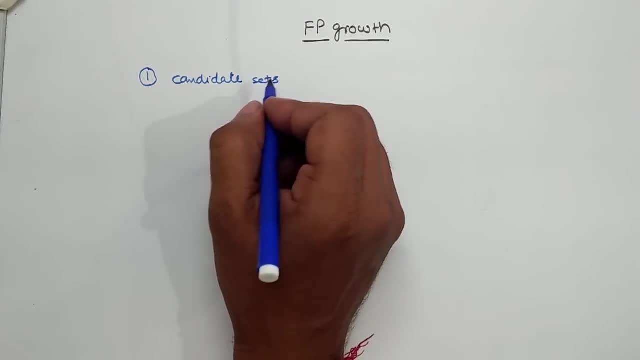 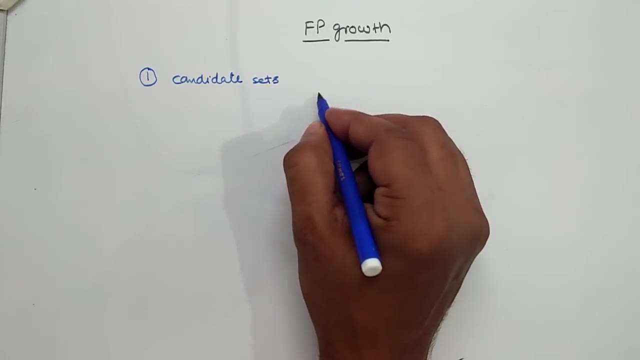 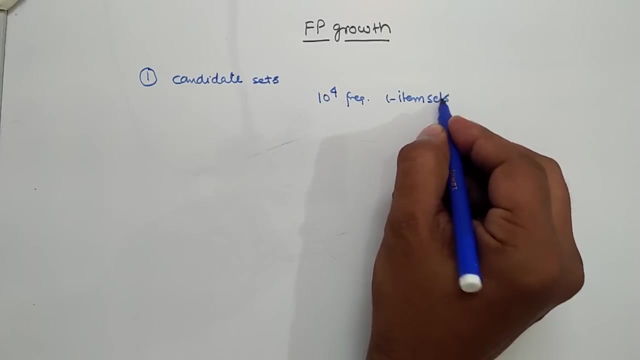 larger in amount, then the combinations are huge and it may, it may be expensive. Okay, So we have to do this operation while we do the computations. So if, for example, if we have ten frequent one item sets in our candidate set C1, then in order to generate a candidate, 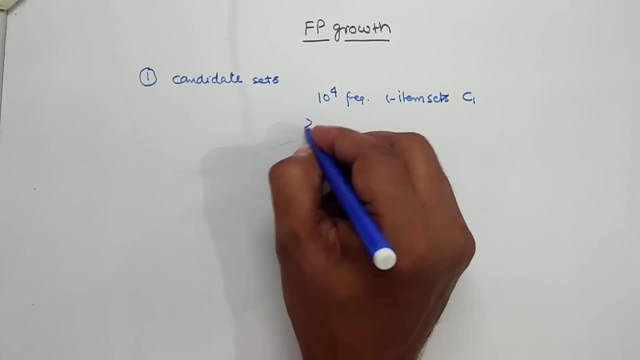 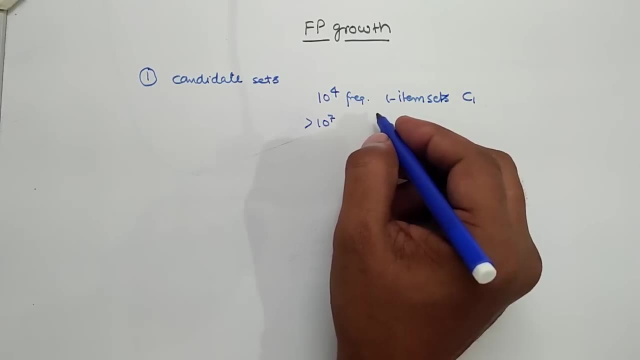 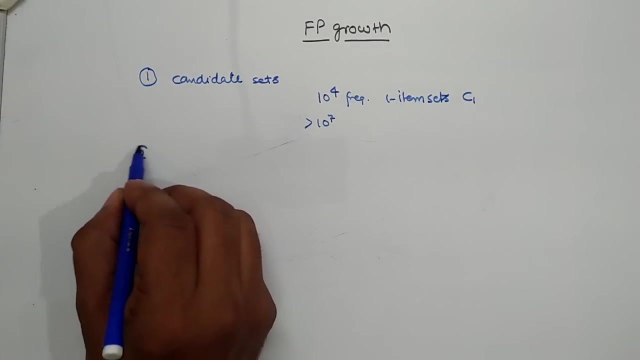 two item set, that is C2. there are something more than ten to the power combinations that is possible. So this is very expensive operation. So at each iteration of a priori there is a process of candidate sets. The second drawback is we have to repeatedly scan the database and due to this it will 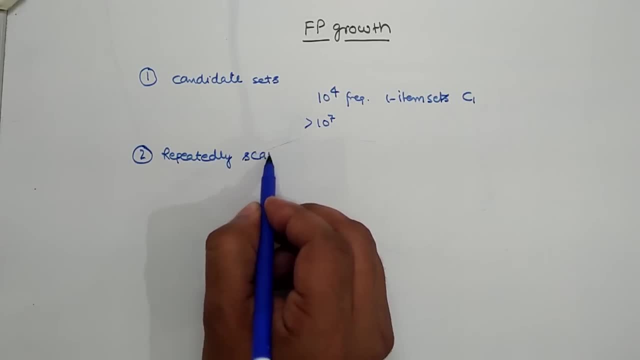 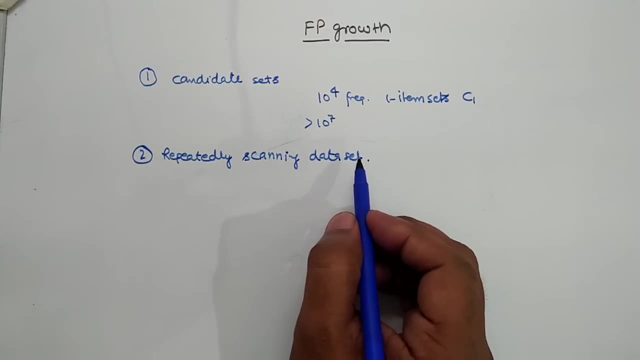 take more time. The process will take more time and the process of scanning the database is very slow. So these are the two main drawbacks which will result in the priori algorithm to make it a slow algorithm. Okay, So we are in the process of finding the algorithm which is faster than the apriori and by which 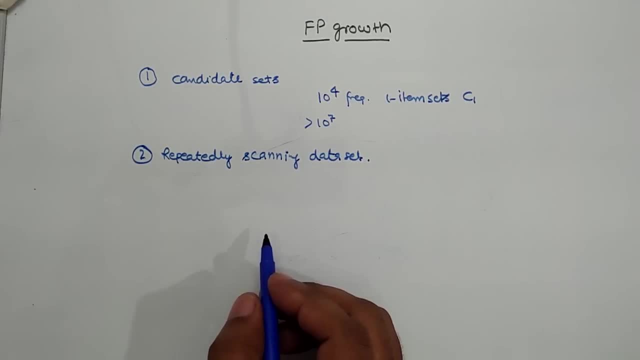 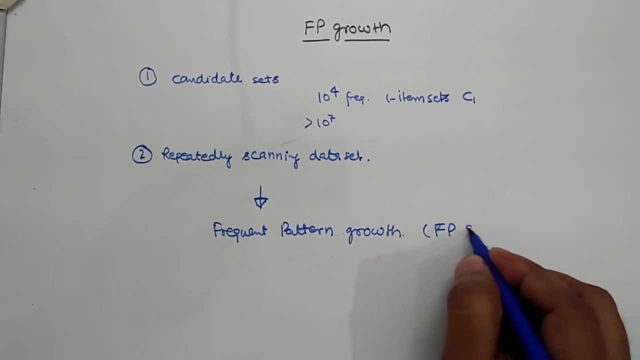 we cannot have to scan the whole database again and again, and we need not to try all the combination of frequent set in order to generate the candidate sets. So the solution of these two problems is frequent pattern growth algorithm, or we can say that this is FP growth algorithm. 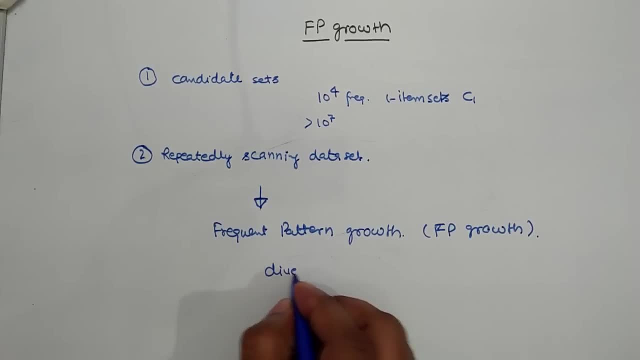 So this algorithm works on the concept of divide and conquer approach, and So the main steps of applying this algorithm includes: first, is it will make an FP tree of the transactional database. And what FP tree FP tree is actually? compress the database, which is provided into a tree form where the node represents the pattern. 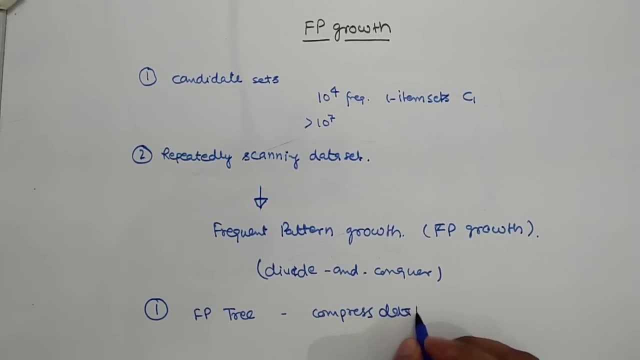 So we compress the database into a tree format where each node of the tree represents the items with their support, or frequency of the item means frequency count, and each branch of the tree represent the association of the item, How this item is associated with the tree. 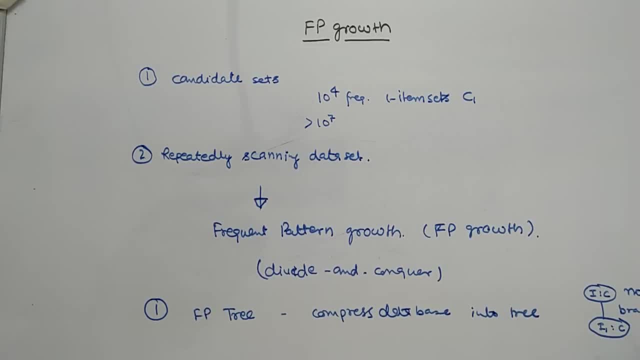 How this item is associated with another item, with the support count. So we convert the whole data set, whole transactional database, into a FP tree. Now, once the FP tree is constructed, then the second step is we have to mine the frequent pattern from the FP tree itself. 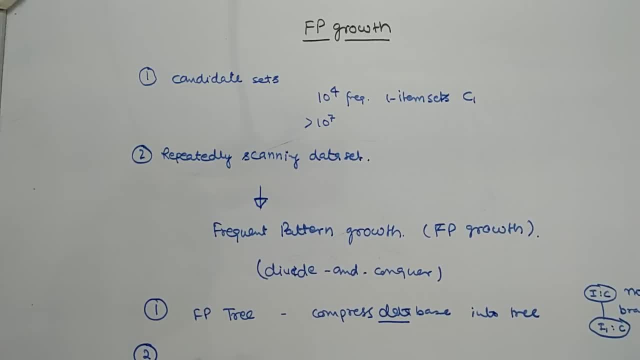 So how we do it? We divide the compressed database into this FP tree. The compressed database is now FP tree. We divide the tree into conditional databases or projected databases, And from those projected databases we have find out the pattern fragment associated with each of the databases. 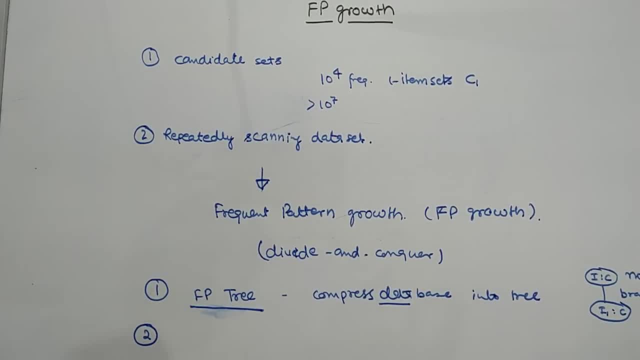 So it is working on something like map. reduce means it will divide your database into different parts. for each part, or for each part of the tree, We have to mine the frequent patterns in that tree. So this is how it will Provide you a fast mechanism to access the data. transactional data. 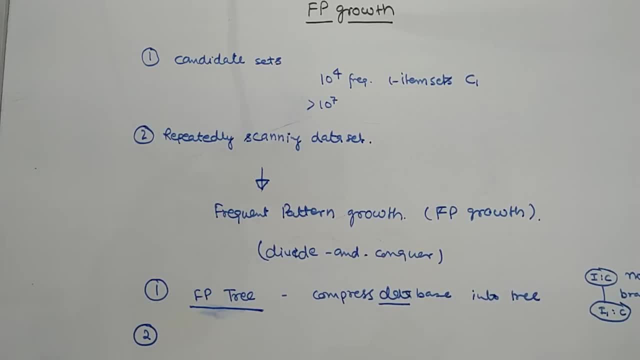 Here we are not required to scan the whole database again and again. Okay, so that's why it reduces the scanning time of database in order of n linear time, While the FP tree is exponential or polynomial time will be taken. So let's understand the FP growth algorithm with example. 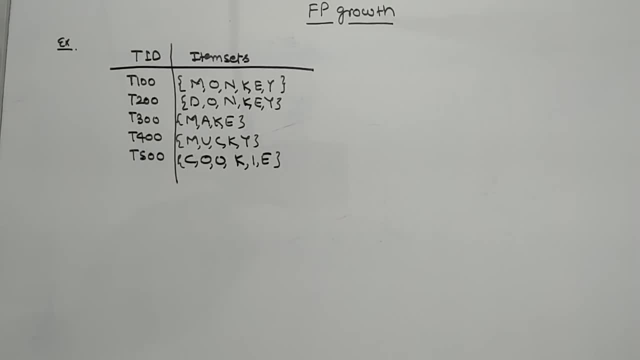 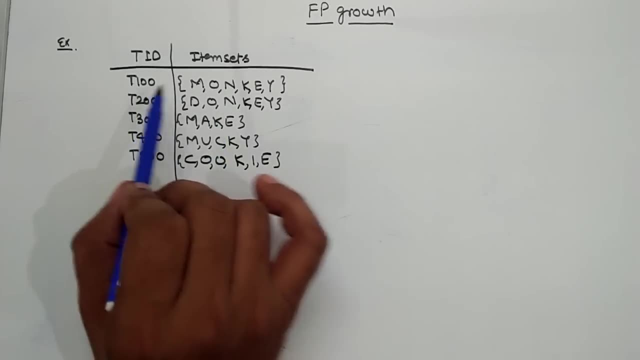 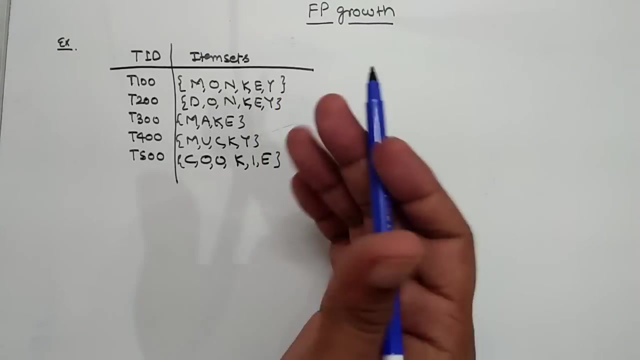 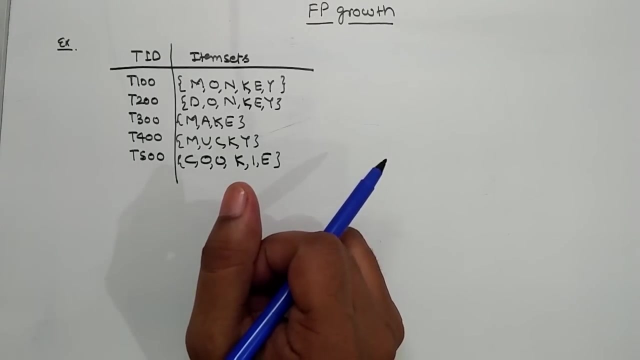 So in this example, five transactions are given in some shopping store and in each transaction some of the items are purchased. Okay, so actually we were in these types of algorithm. We want to find out the association between these items, like, for example, if you are purchasing something from Amazon or Flipkart and you are providing some suggestions. 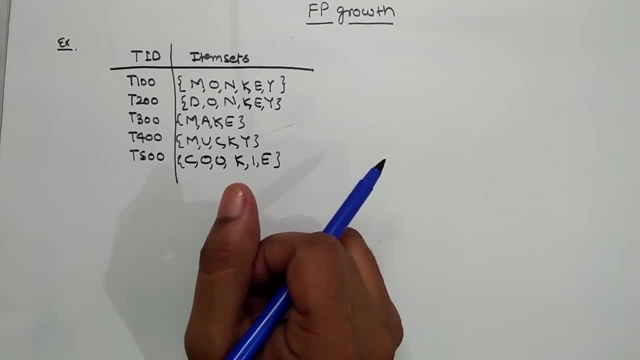 Regarding the product you are purchasing. suppose you are purchasing a mobile and some suggestions are provided to you, like a mobile stand holder, mobile cover or the screen guard. so these items are actually presented by some of the analysis done based on the customer transactions, previous customer transactions. so here we are, finding the similar analysis we want to. 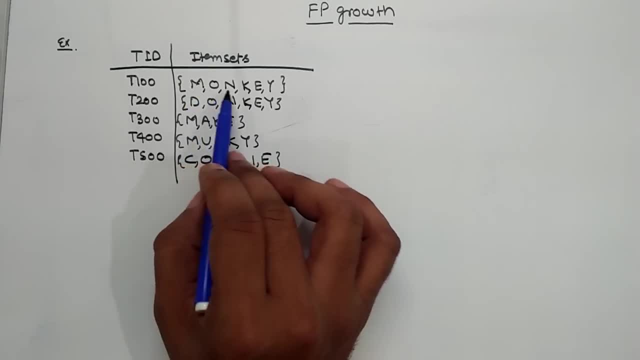 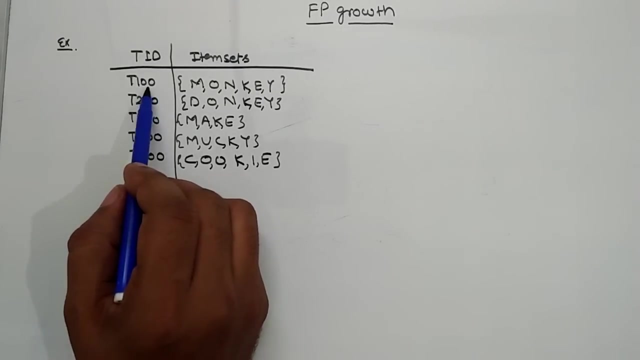 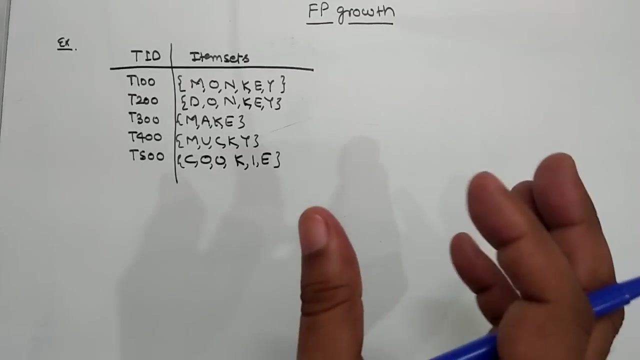 find out the associations between the purchased item by the sum of the transaction by some of the customers. okay, so in this example, let's suppose M is some item purchased in, purchased in transaction, this transaction ID T100 by some customer. okay, and the outcome of this algorithm is to have a frequent patterns or association rules by which we can say that. 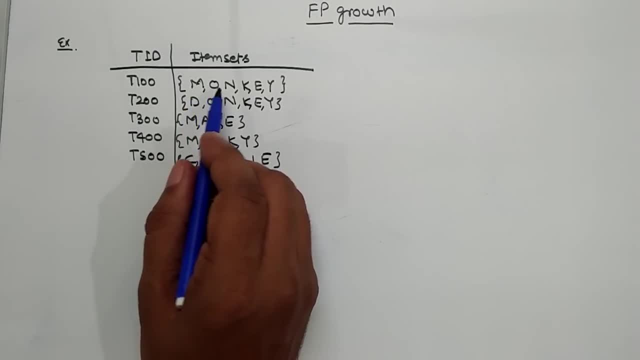 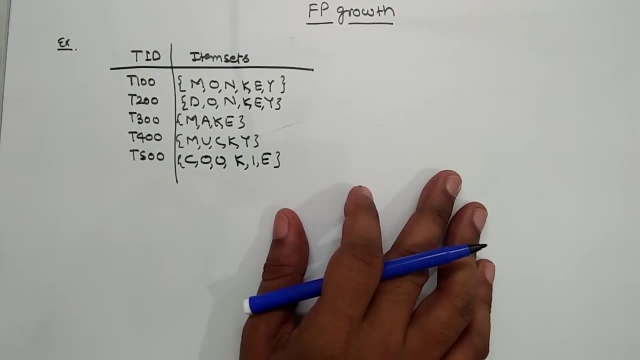 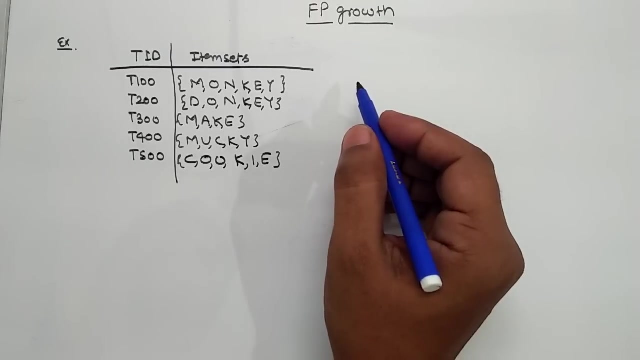 if someone purchase M, then what is the probability of he would purchase O? okay, so these are the some of the intuition behind the reading. these algorithms now move. come to the point of FPGrowth algorithm. now, the first step of a FPGrowth algorithm is similar to the a priori one. we enlisted the number of 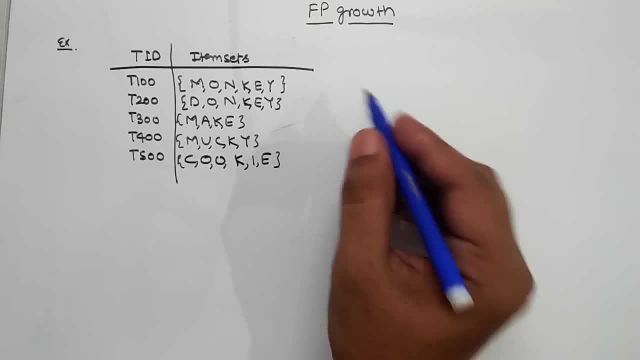 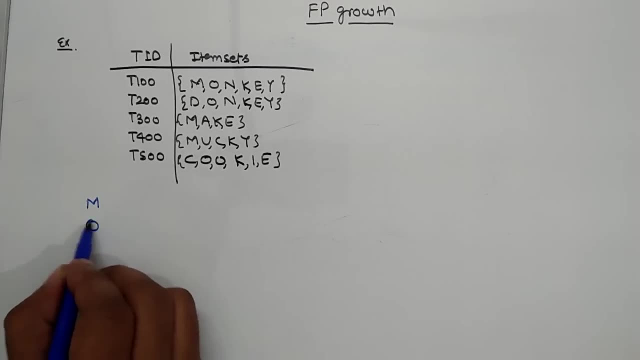 items presented in the transactional database. so here that we enlist the number of items we have M, K, E, Y, B, A, M, M, A, M and I. so these are the items which is there in our database and we have to write also the support count for each item. we have to scan the database and write the support count. 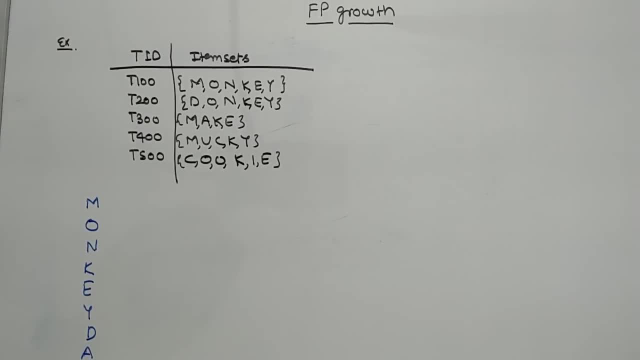 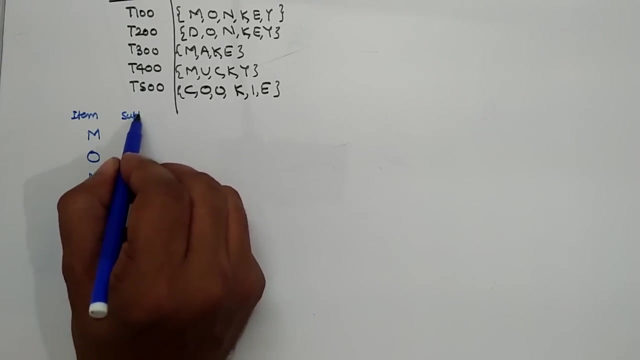 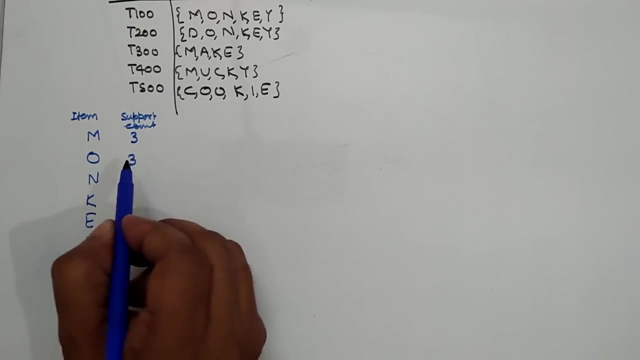 Centerione and Jewish M, m, o, E, e, the o. So the support count for M is 3,. you can check the database. support count of M is 3, support count of O is 3, for N it is 2, for K it is 5,, for E it is 4,, then for Y it is 3, for. 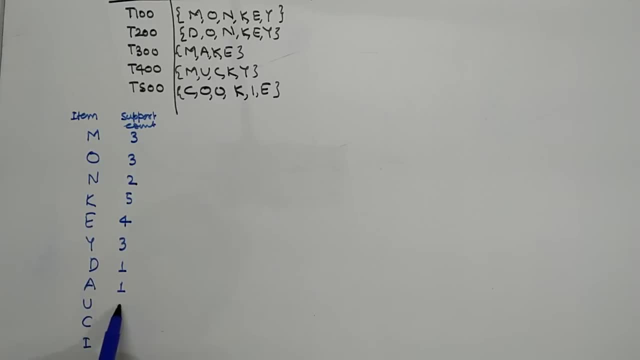 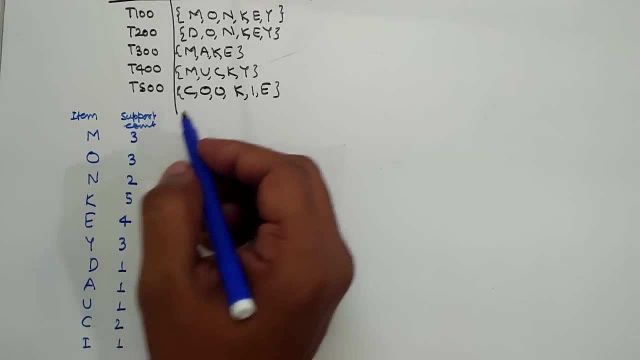 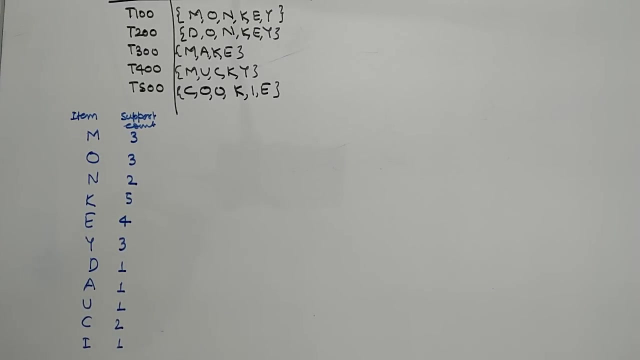 D it is 1, for A it is 1, for U it is 1, for C it is 2 and for I it is 1.. Now we are also provided minimum support for each of the such type of questions. So for this one suppose, the minimum support which is given is 3.. 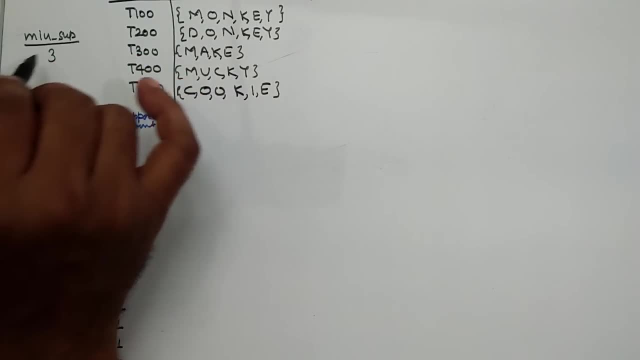 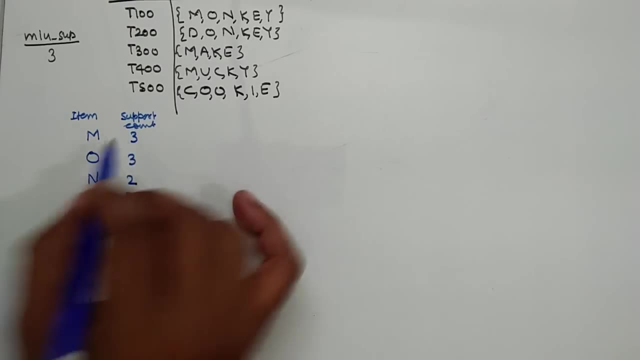 So the minimum support for this transaction is 3.. So we have to analyze the data based on this minimum support, 3. So this is our item set. then we have to find, based on the minimum support, we find out the setup. 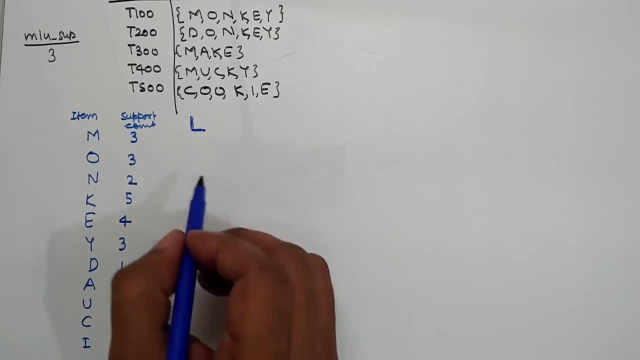 Set L, which only contain the frequent patterns or frequent items. So frequent items are those items whose support count is greater than the minimum support. So we can reject these items from our table because they have the support count less than 2 and write down the items in decreasing order of support count. 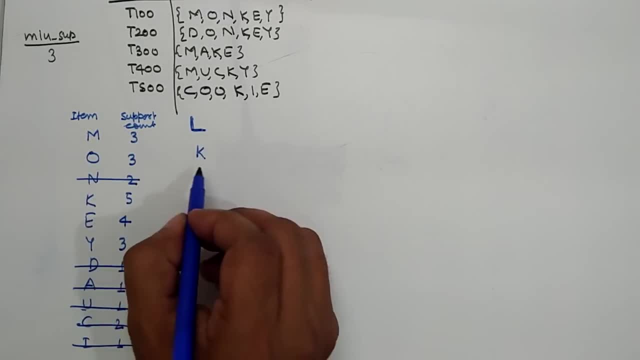 So the maximum support count is K, Then second is E, then we have M, then O and Y. So these are the items and their support count is for K I 5, for E 4, M is 3, O is also 3. 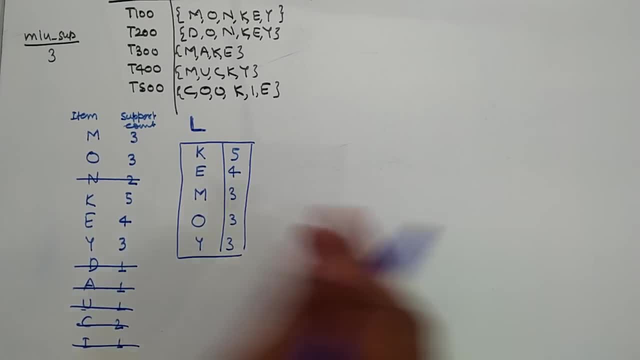 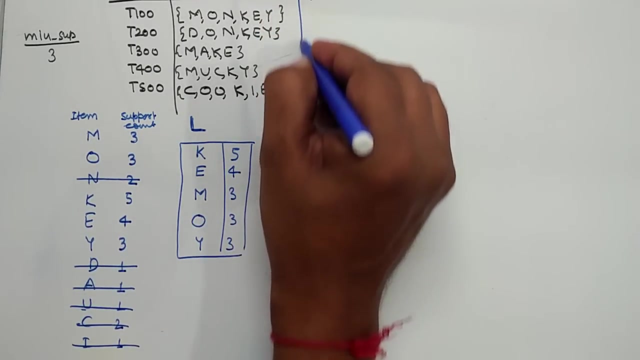 and Y is also 3.. So this is the first two steps We have. We have only scanned the database only one time until yet. After that we have to construct FP tree from this transactional database. So in order to construct the FP tree, first we have to find out the ordered item set based. 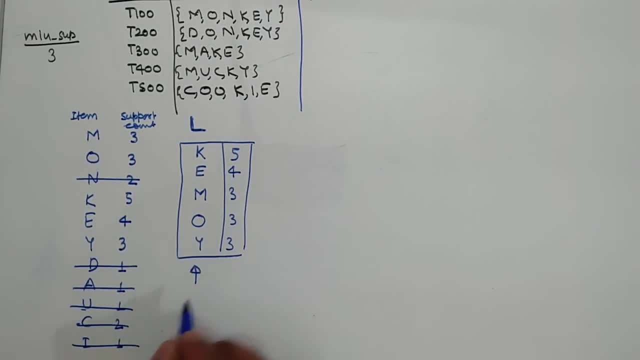 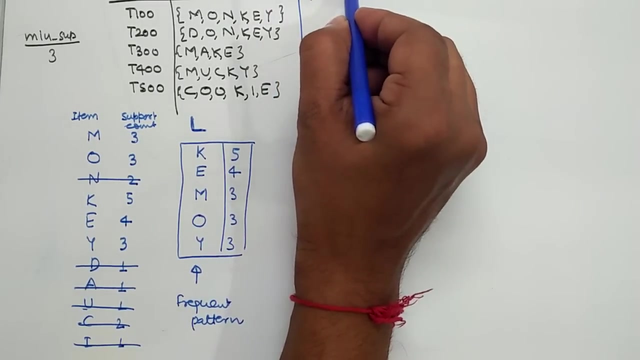 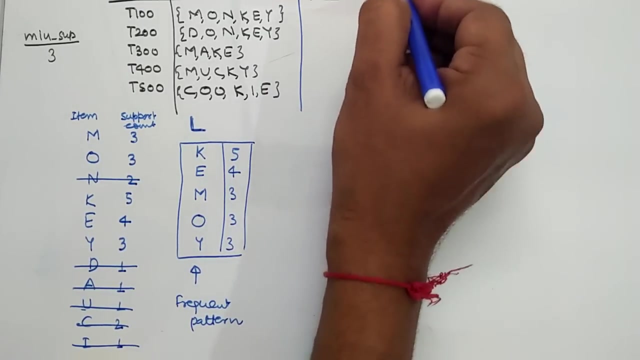 on the pattern which is provided here. So this L is also called frequent pattern, Frequent pattern. Okay, So this is the initial frequent pattern And based on this frequent pattern we have to find out the ordered item set. Okay, So how we find out the ordered item set. 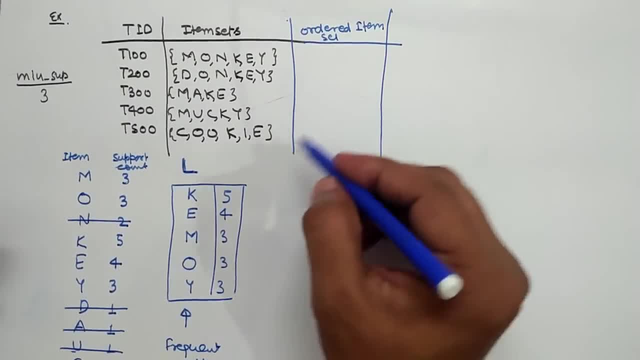 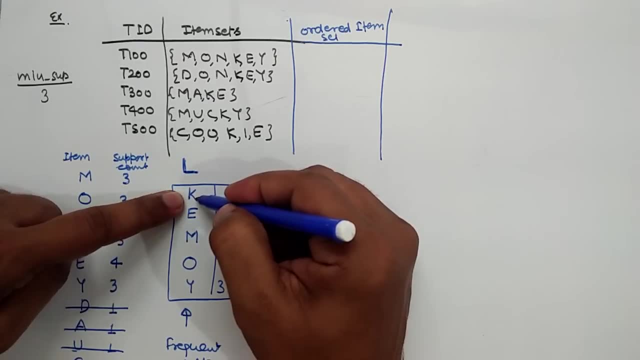 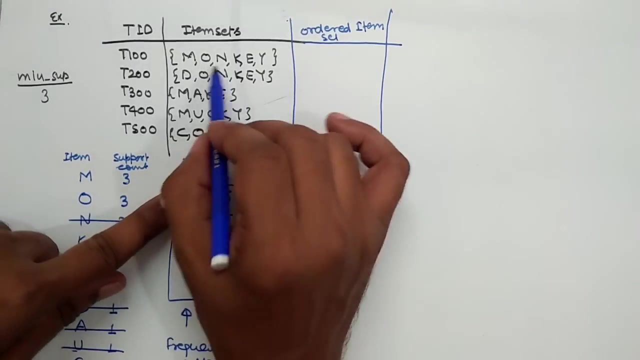 It is very simple but we have to do. we just scan each transaction based on this pattern. So we have to find out pattern one by one from the transaction and write it here How we do it. For example, we have to check for the K in this transaction. check for the K. K is there. 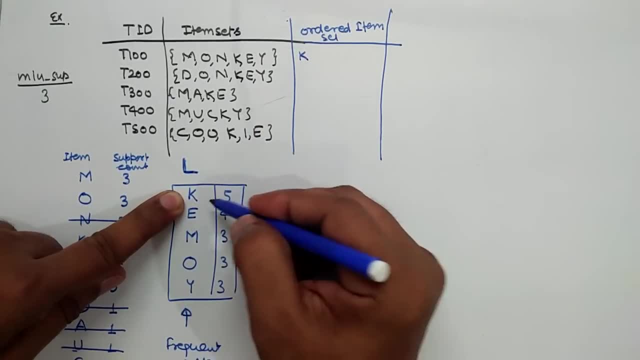 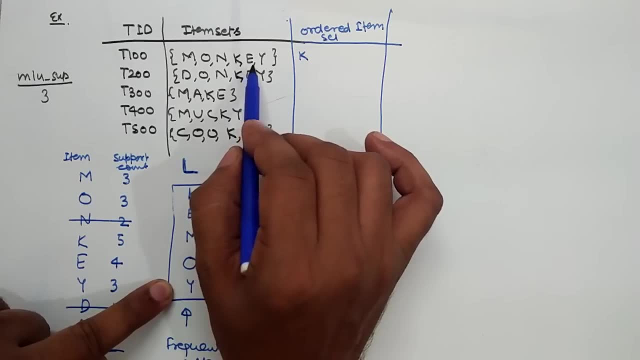 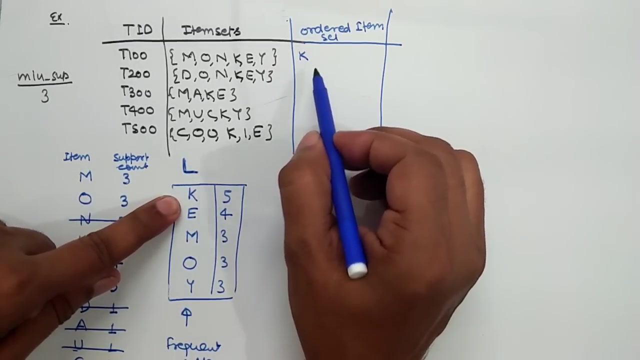 write the K. always remember that you have to write the ordered item set according to this pattern, not according to the order which is given in the transaction. Okay, So first we have to write K, because K is appeared first in the L set. 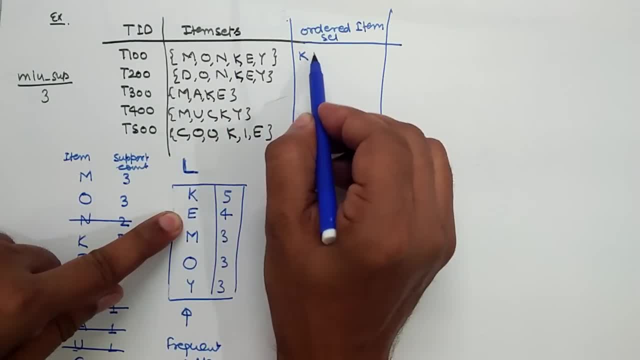 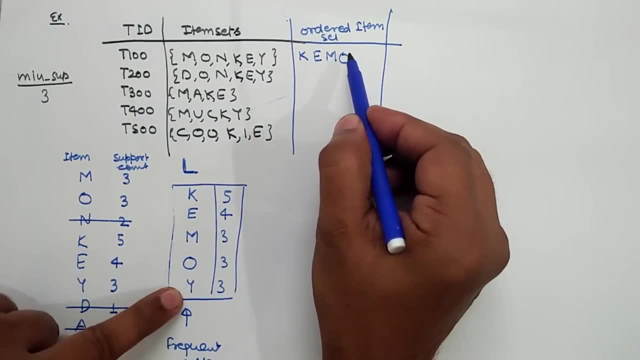 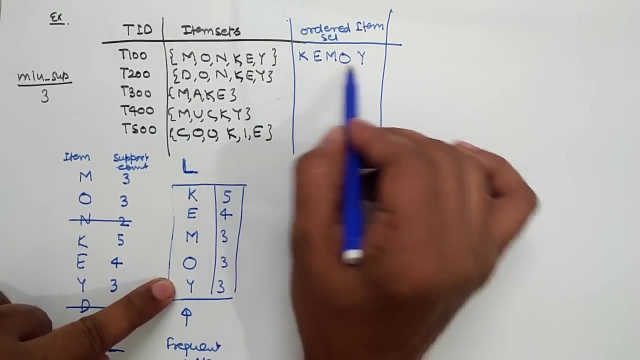 Then we have to write E. if E is there, Yes, E is there. We can write: M is there, Yes, M is there. We can write: O is there, Yes, Y is there- Yes. We find all the items in the pattern in the first transaction and we write these item. 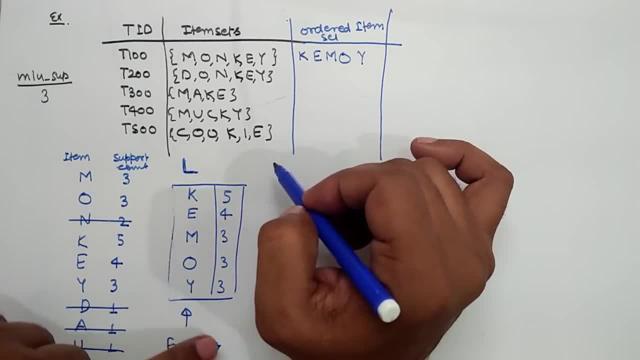 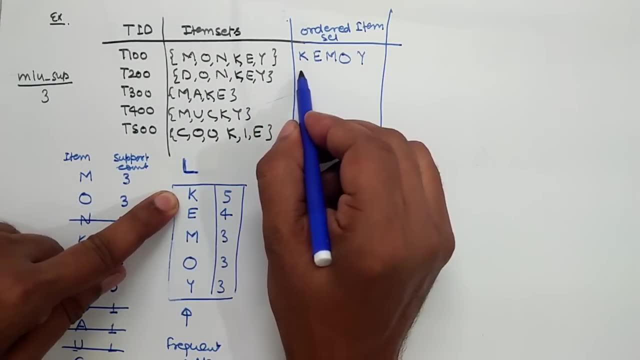 in the order of the decreasing order of frequencies. Okay, Again, we do the repeat the same process for transaction 200.. So K is there, Yes, E is also there. M is there, Yes, M is not there. Here, M is not there. 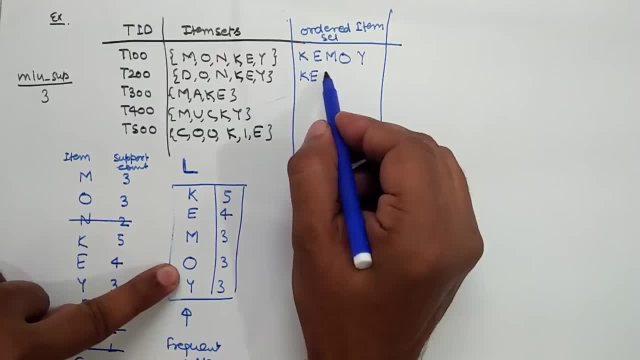 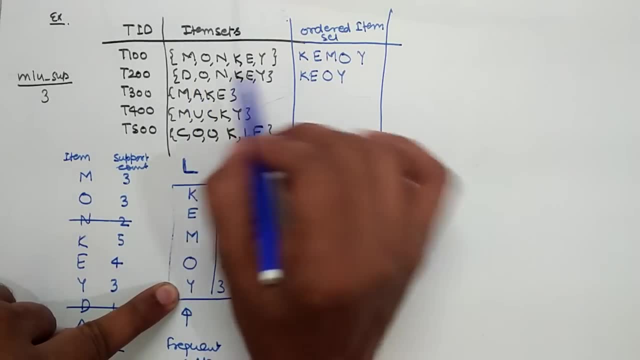 We are not writing here. M O is there, Yes, Y is there, Yes, Just it, Leave it. We do not want to write D and the remaining items of this transaction. Okay, We have to write only those items which are in our treatment pattern. 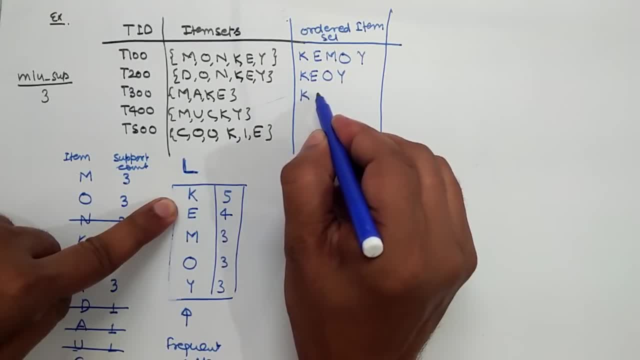 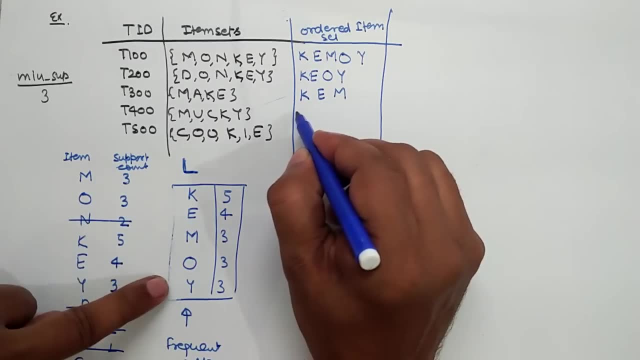 Then for third transaction, write here: K, then E, then M, M is there, Yes, Okay, Okay. So K is there, O is not there, Y is not there. For fourth transaction: K, E is not there. 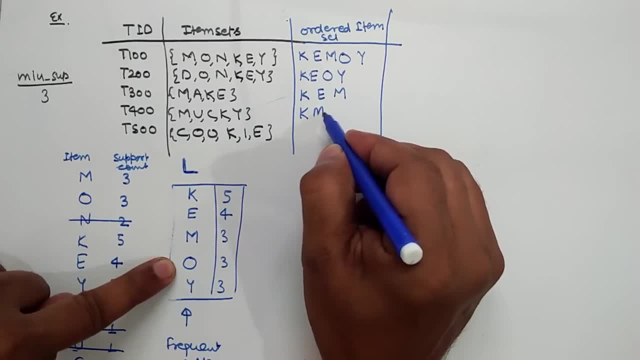 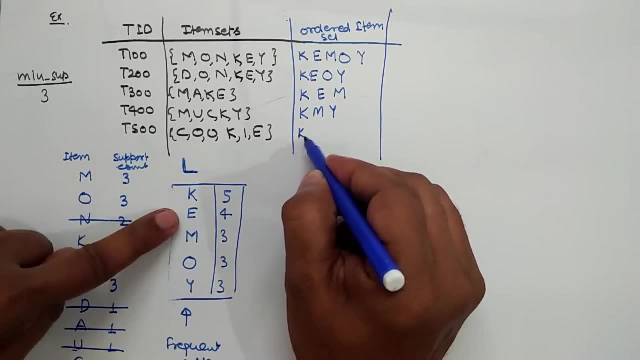 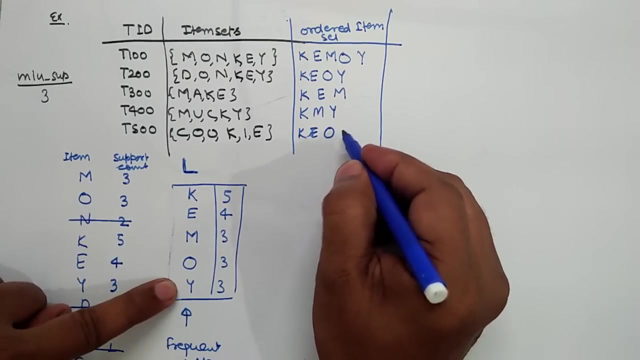 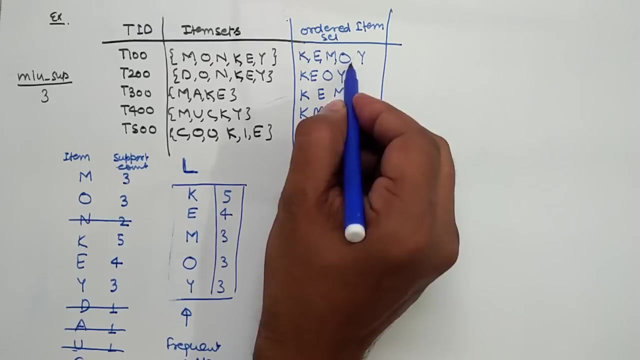 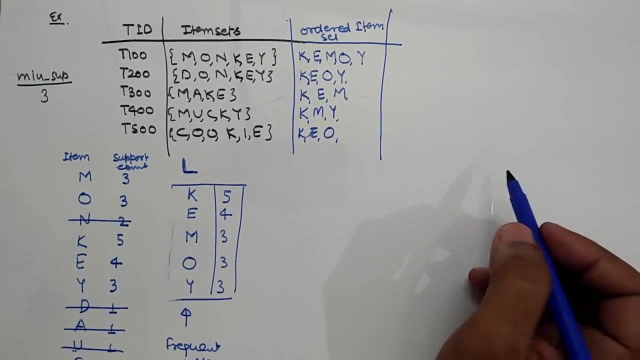 M is there. So K, M, Then O is not there, Y is there. Yes, Again K, then E is also there, then M is not there, O is there and Y is not there. Okay, So these are the ordered item set which is found from based on the frequent pattern in the first step. Okay, So now we have to construct the tree. In some of the book textbooks we can construct the tree directly, but it is easy that first you write the ordered item set. based on these ordered item set you have to make the tree. Okay, 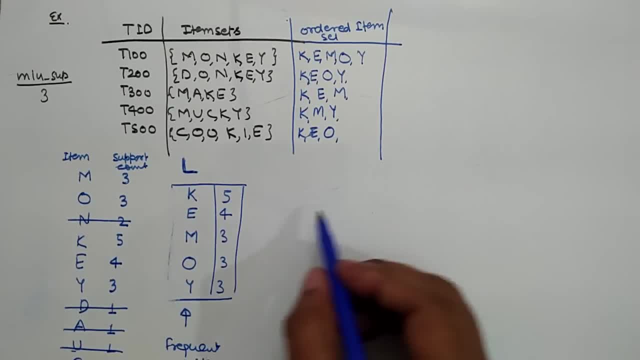 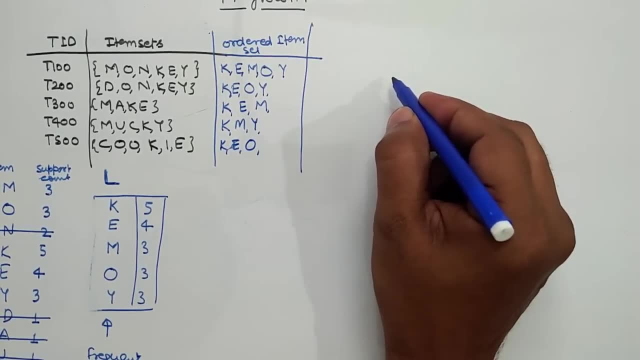 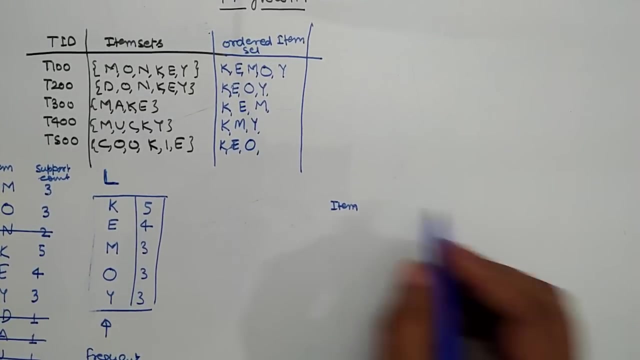 So for tree construction we make a, so suppose I draw the tree here. So first we make the table of the pattern here. So the table is we have item, item ID. So it is K E M O. 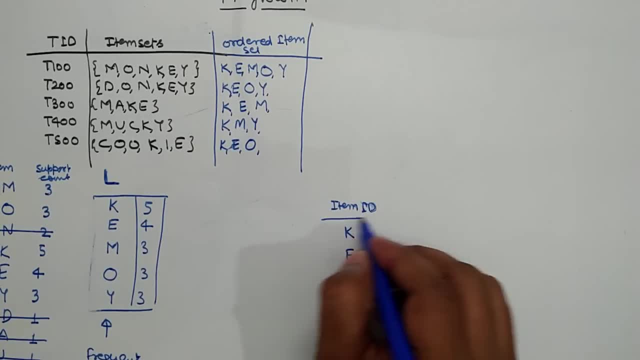 In the same order, in decreasing order of the frequencies. then we write the frequencies of each item ID. Okay, So the frequency is 5, 4, 3, 3, 3.. And so this is a support count for each item ID. And in the last we provide the node link to the tree. Okay, 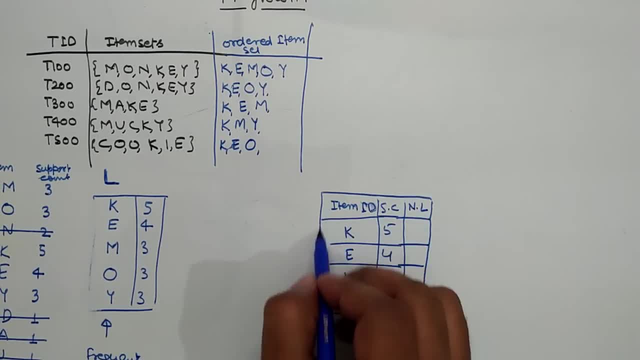 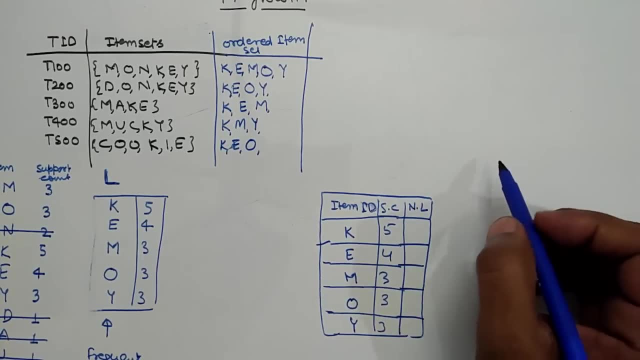 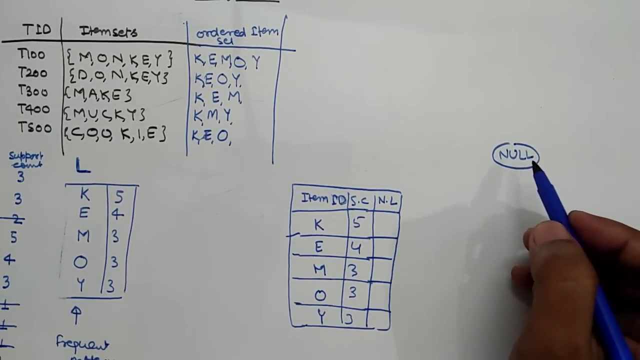 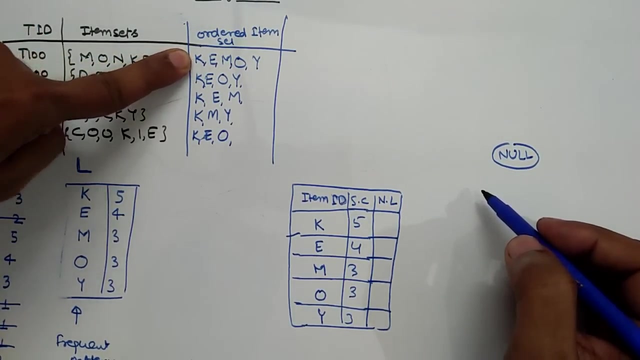 So this is this table, So the node link can be treated as a header of our tree for easy traversal. Okay, So start with the tree construction. First step is make a root which is empty or null, Then draw these ordered item set into the tree. So first we have to draw for the transaction T100.. First item set is K, So the node of tree is a item set with the frequency count. 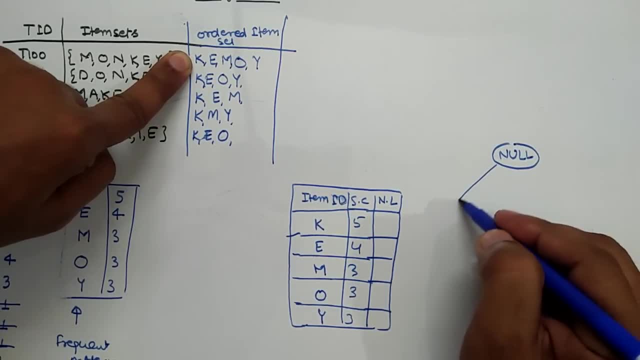 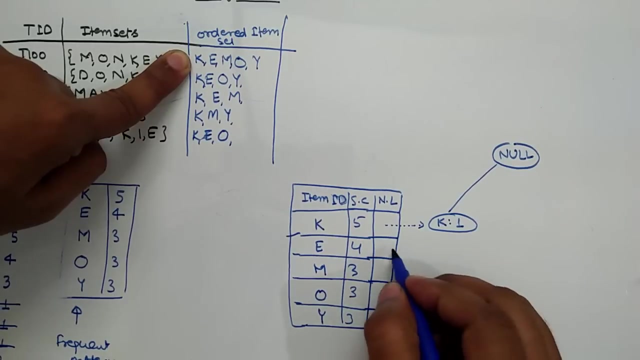 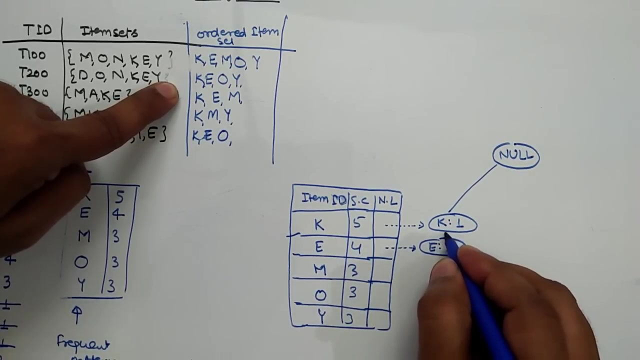 And the branch is the association between them. So the first is K, So we fetch the K and draw a node with the K count. We have taken only one K, So K with the support one. Then we have to draw E, because second item is E in this transaction, So E with the support one. we have to link those items. Then we have M. 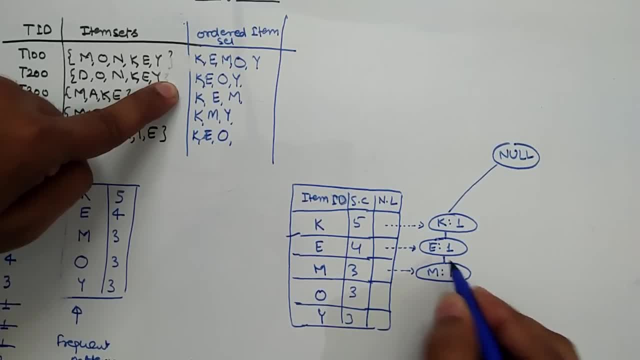 So we draw M here with the support count one, Then we have O, O with the support count one, Then we have Y. We have Y with the support count one. Okay, So here we have. draw the first transaction. Similarly, we can draw the second transaction as K again. So because K is repeated, we can draw the second transaction as K again. 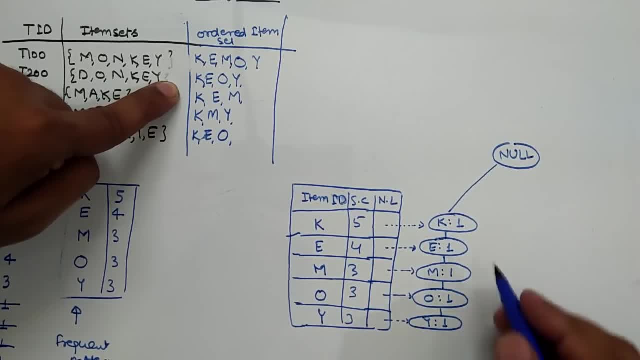 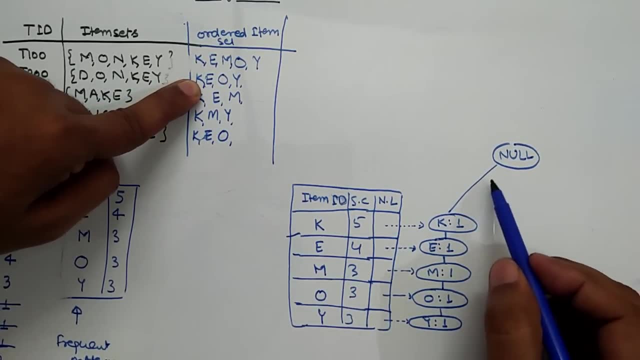 with the support count one. okay, so here we have. draw the first transaction. similarly we can draw the second transaction as k again. so because k is repeated, we can increase the count as two. then e is also repeated, increase the count as two. o. so we are not find here o, so we make another. 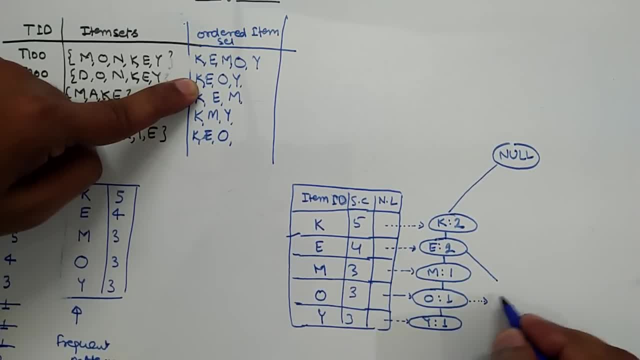 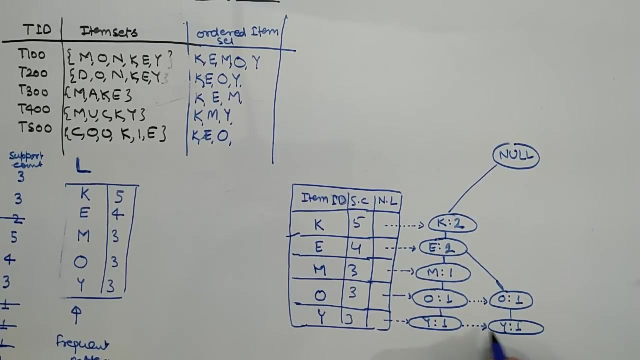 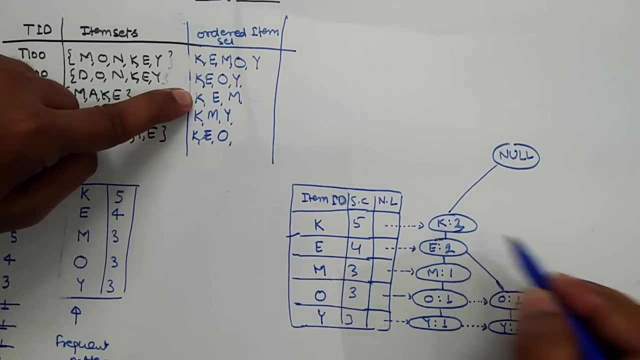 branch and draw the o item with the frequency. okay, then after all we have y, so draw another y with the frequency count and link this y with the previous one. okay again for the transaction, again k, so k is now three is also three and m, so m is the first function of the second part. so 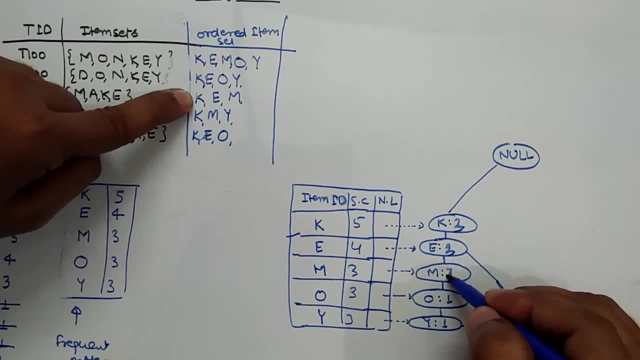 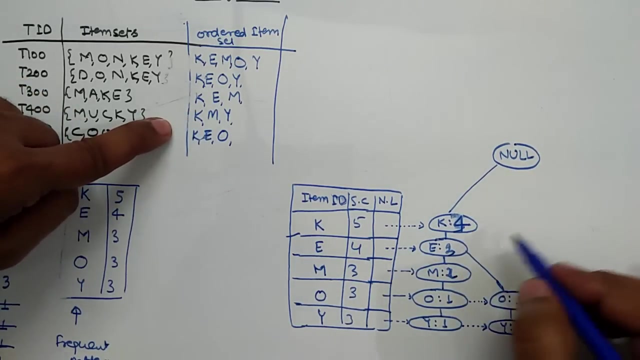 is also 2, so make here 2. that's it. then again k, so k become 4 after this. so i just make here 4, then m. m is not there, so we have to make another m, like this m with frequency 1 and link with the previous node. okay, then y. so after m we found y item. 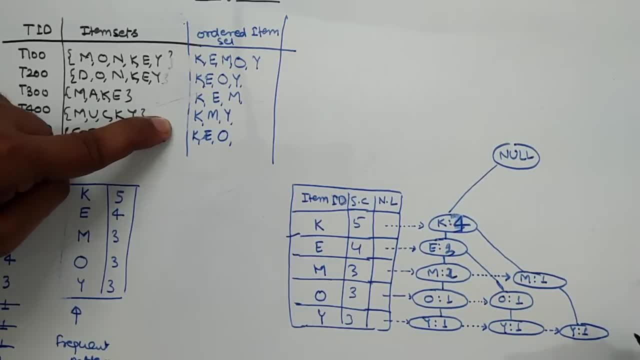 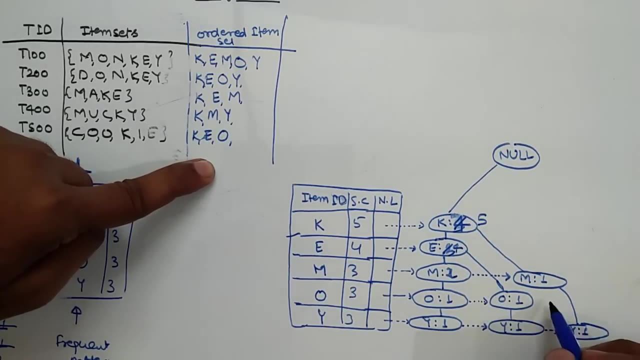 so this is y link with this one. then again k, so k is now 5, e is now 4, then o, so o is not there, so we make another o here, so make another o, like this o with 1 and link with this previous item. 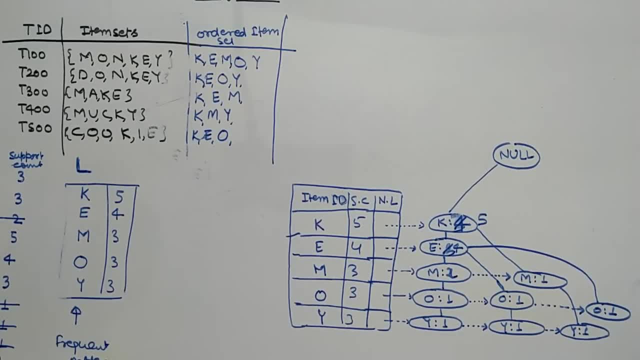 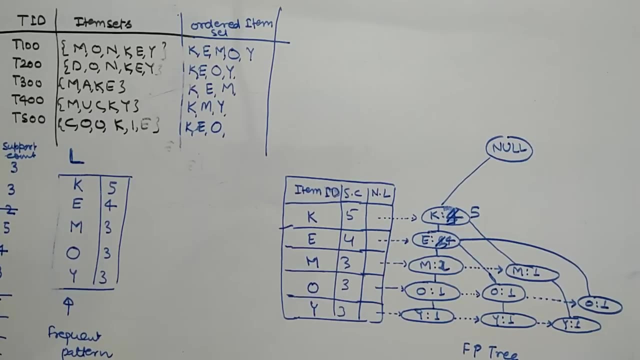 so this is how you construct the fp uh tree for the uh from the transaction database. this is known as fp tree. now, from this, this is the first step of their fp growth algorithm. how to construct the fp tree. now, after this, we we have to make find out the conditional. 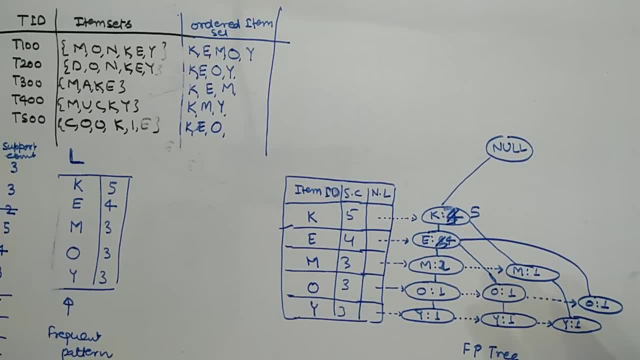 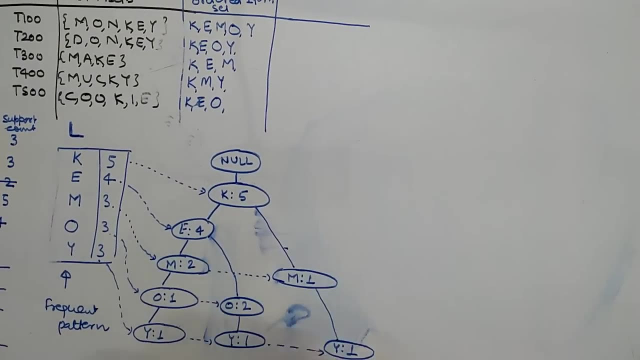 pattern base and based on conditional pattern based, we have to find out the conditional fp tree and then we have find out the frequent patterns. okay, so let me make it clear for you so that it is easy to understand. so once you have drawn your tree, then we have to write the items that is on our pattern in the reverse order of the frequency. so we 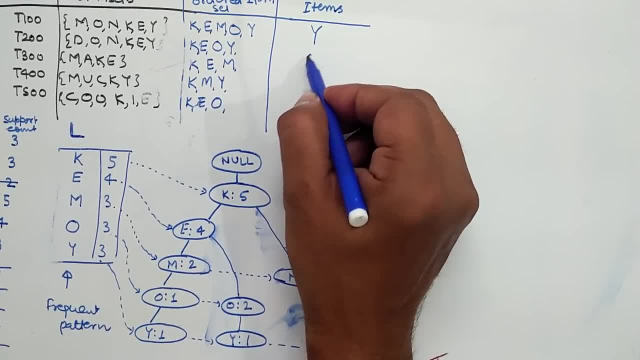 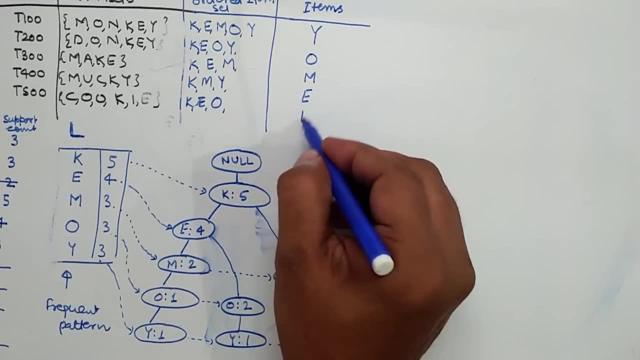 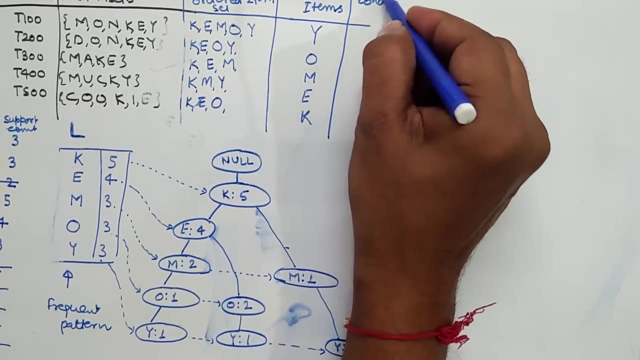 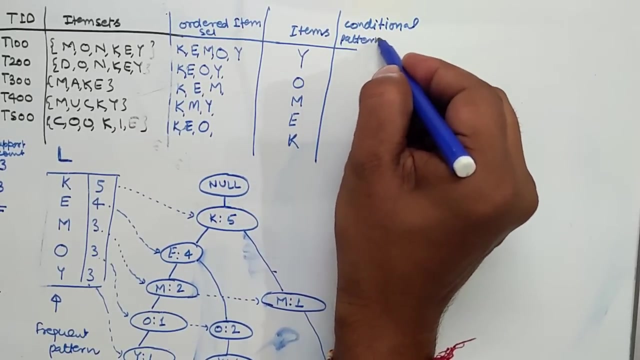 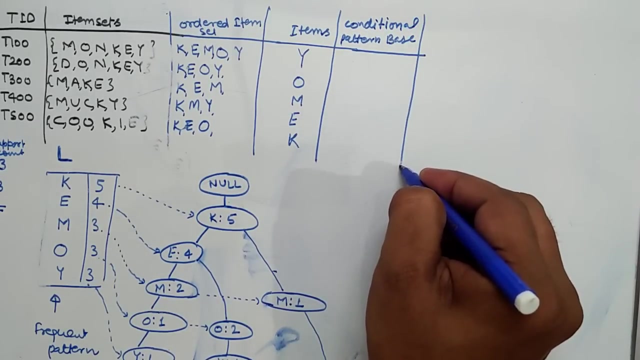 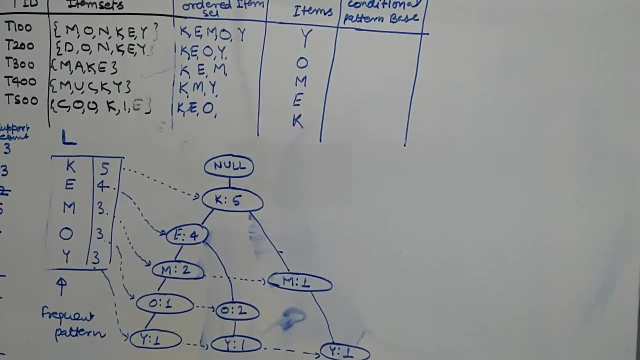 we have to write Y first, then O, then M, then E and then K. based on each item, we find the conditional pattern base. conditional pattern base: what is this conditional pattern base? it is the individual path by which we get these items. so we have to find out the paths of Y in this FP dragon so we can see that. 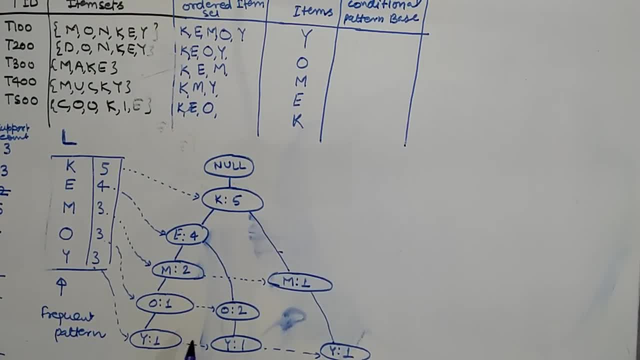 Y is achieved here by three paths. so we have to write all these three paths here and the count of the y which is achieved by each individual path. so so, for example, Y is achieved by this path and so we have to write this 3 path below and we have to write this wealth path and this 8th 1 road. so we have to start from each place by which we have Beast week, the common process with each class, with Y, and how the log and others, then their pattern, satisfied by each particular value of this alone, No limit. 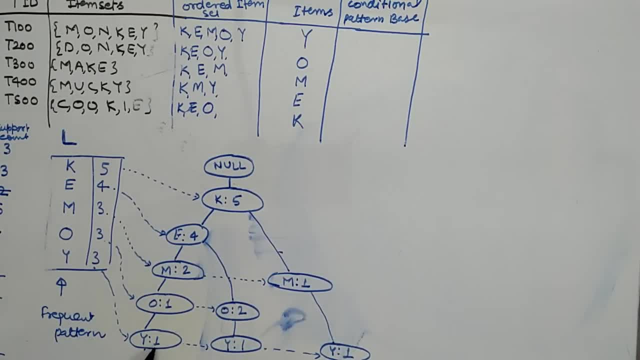 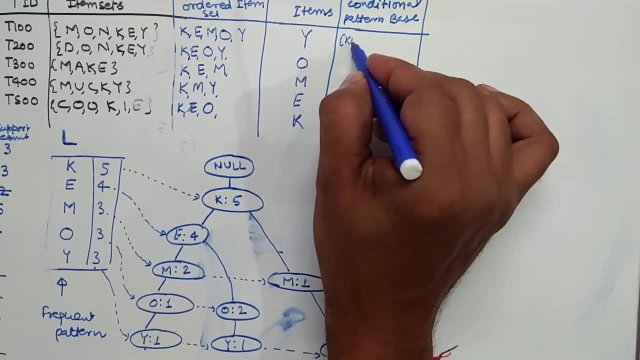 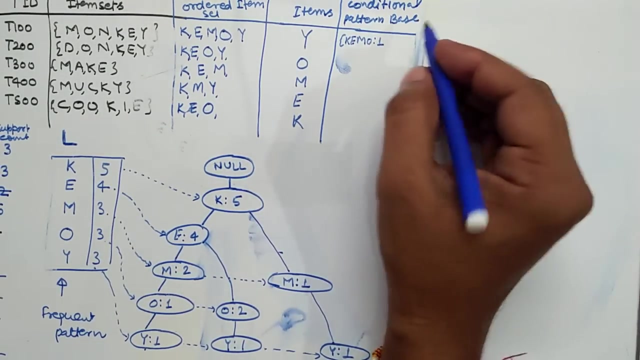 K E M O and we found Y as support one. so I write here K E M O with support one. similarly I write K E. sorry for this one, so I just extend this line little bit. okay, so I write here this one. and second part is K E O with support one. and third part is K M with support one. 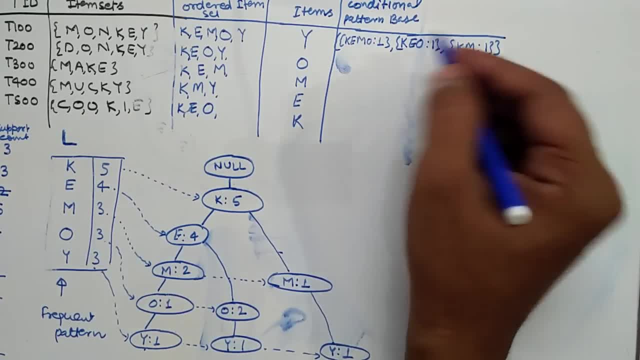 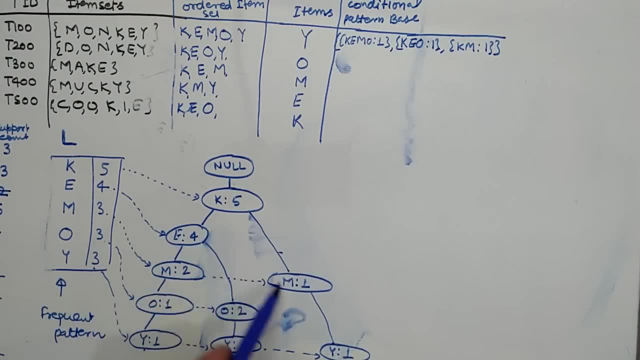 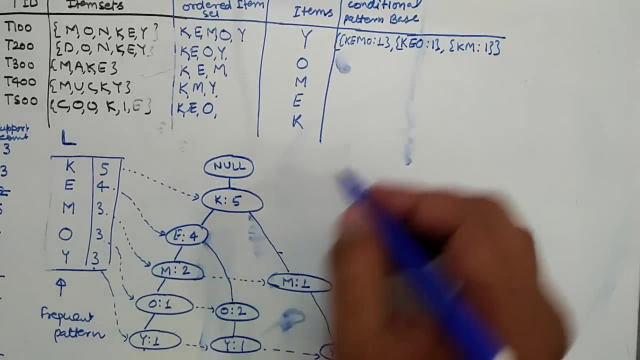 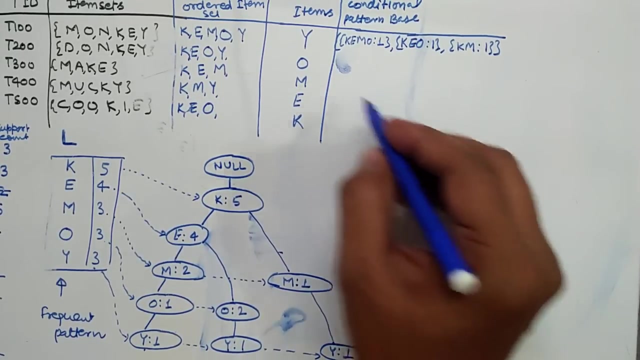 so these are the three conditional pattern base which is found for Y. okay, so I think easy to visualize K E O, second one, K M, third one, and the frequency or the support for Y is one In all cases. similarly, for O O is find out by two paths. one is K E M, so K E M with support. 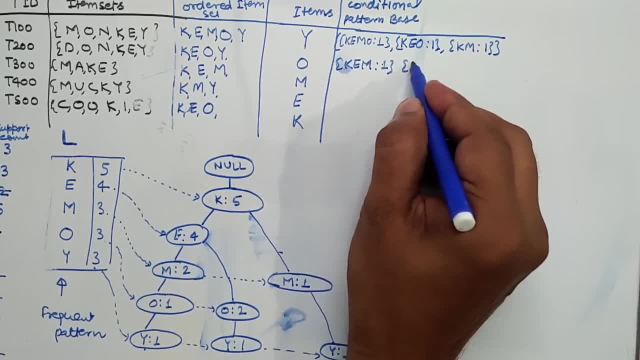 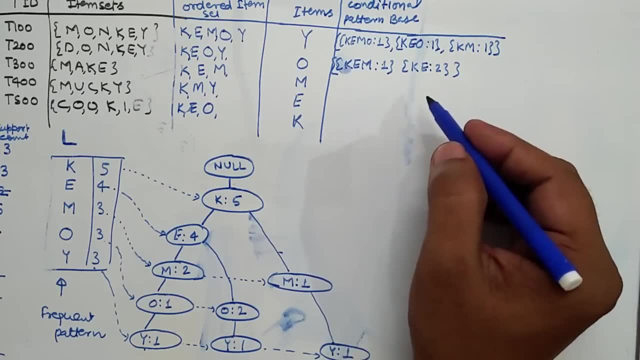 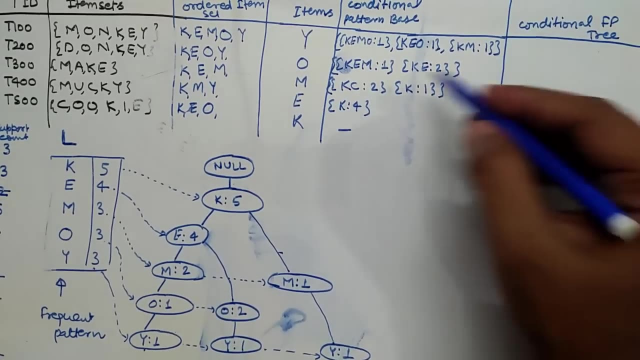 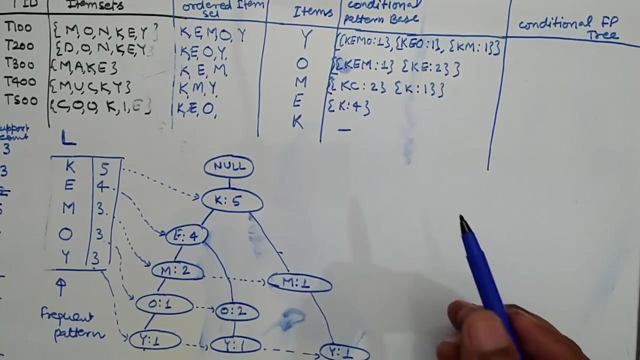 one and other is K, E with support two. okay, so this is the pattern base of O. similarly, we write the pattern base for all the item sets. so we have written all the cases. for K, it is empty because we do not find any path to reach K. K. the previous node is root node, which is null. now when, while you constructing, 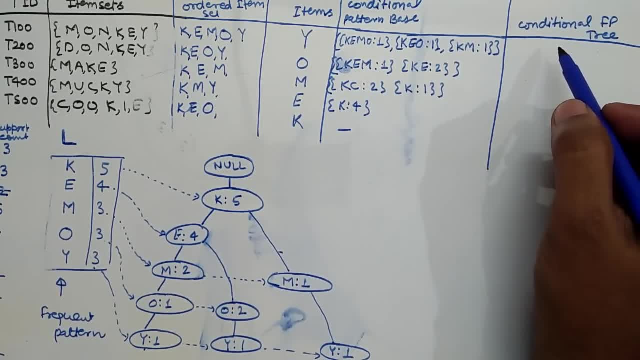 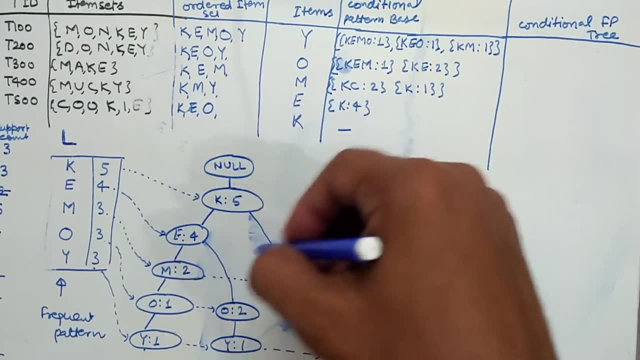 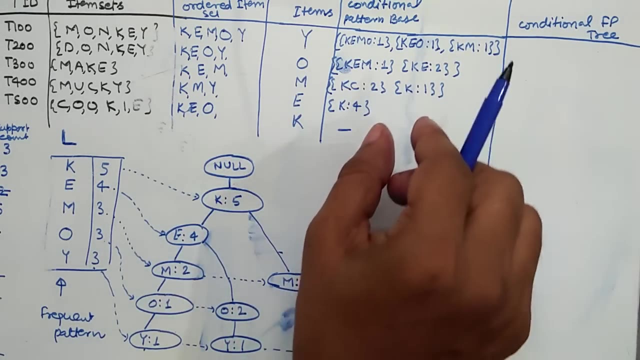 the pattern base. the further step is to construct the conditional FP tree for each of the item set. now we are dividing our whole transactional data. first we divide the whole transaction into FP tree. then we have find out the conditional pattern base For each of the item. then we divide this into a frequent pattern trees. so for each of this, 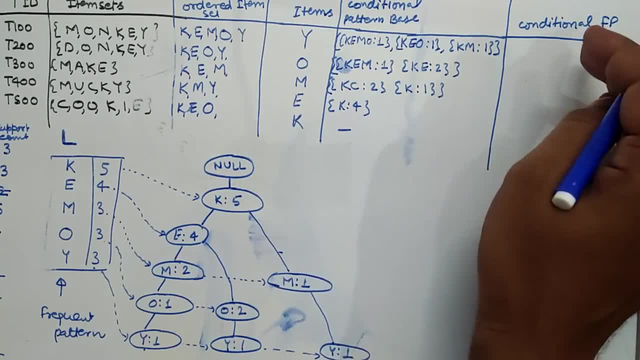 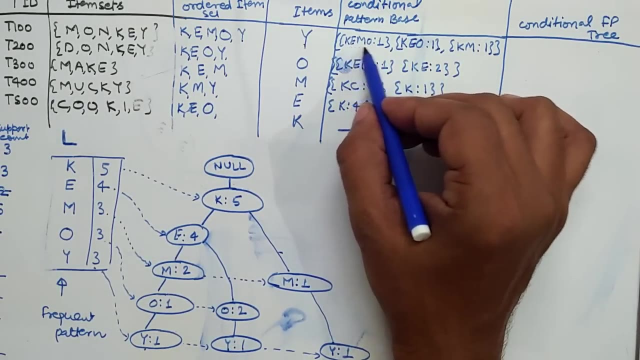 reduced or frequent item base. we construct a conditional FP tree for each item. so we have to construct the conditional FP tree for Y and how we do this? we have to find out the common items in these sets, all sub trees. so for these three sets the common item is only: 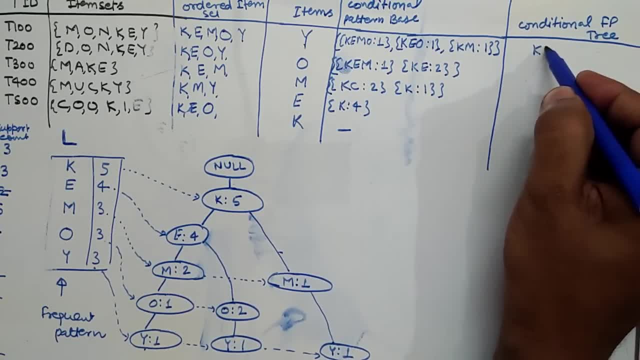 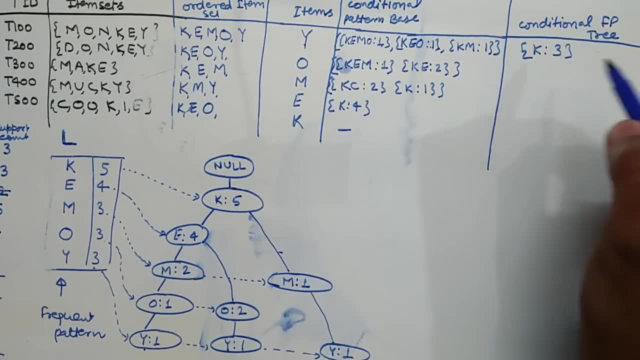 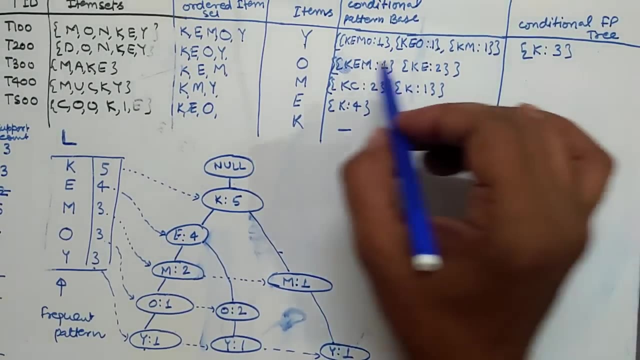 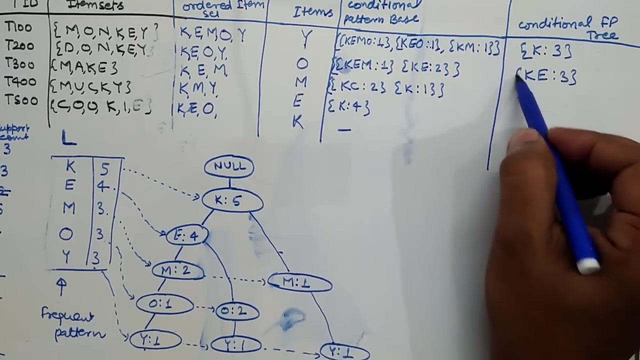 K. So we write here: okay, and count of K is 1,2,3, summation of all these sub trees. so this is one sub, one conditional FP tree for item Y. similarly we find out FP tree for item O. so the common at attribute is K, E, with support three. then in this one it is only k will support. F and in this one it is same K. So we write here: okay, and the count of K is 1,2,3. summation of all these sub trees. so this is one sub, one conditional way, an. in the last we found out that joint tree for item. 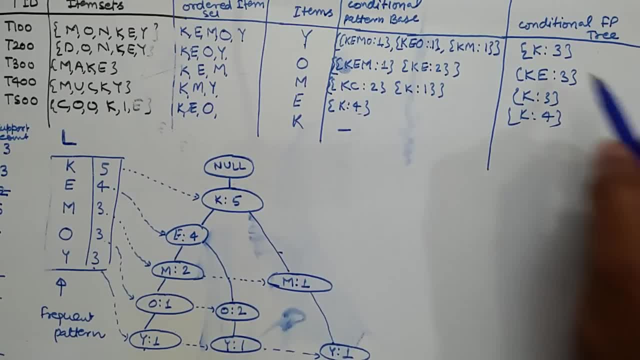 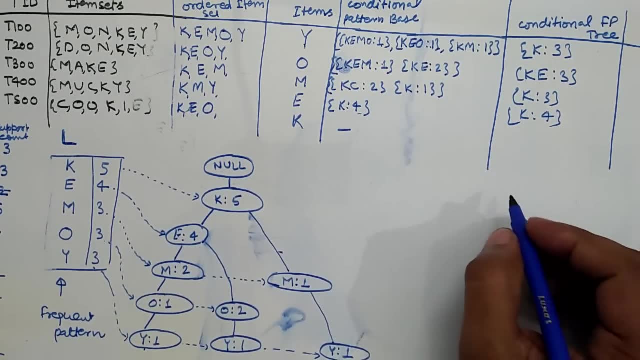 O for symbol, or first item three, which will- Tommy, it is few. symbol one: use a variable four. okay, now, while you are generating conditional fp trees now, next is the final column and which is known as frequent patterns. so this is all you need to be derived, frequent patterns generated. 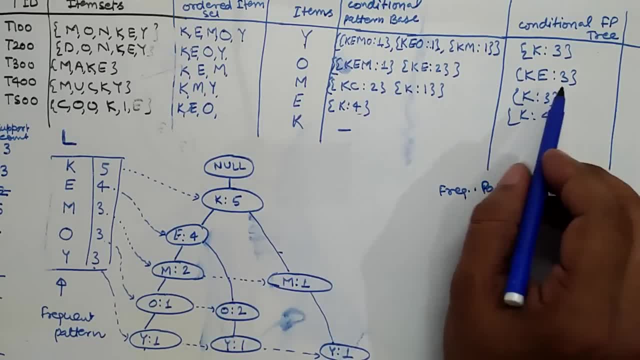 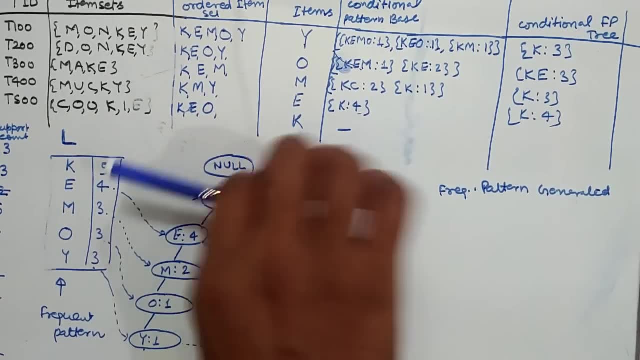 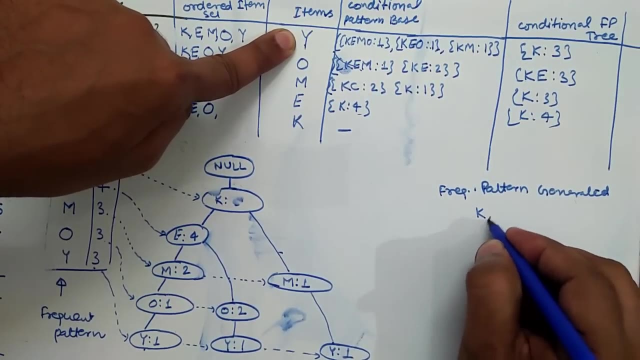 so how we generate frequent patterns. from this conditional f3 we find out the combination of the item with the fp tree. so for so, sorry. so for this one the conditional pattern would be formed as ky, k in combination with y, and the support count is 3. this is one frequent pattern for this. 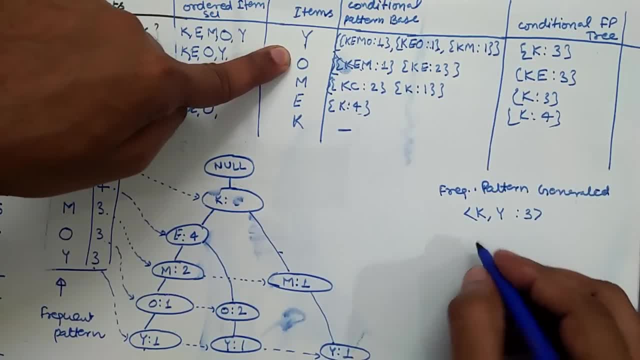 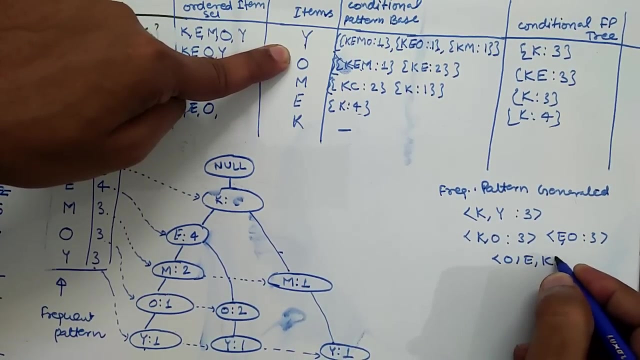 item set because it contains three items. so all combination would be there in the frequent item set, that is ko, and with frequency 3, e, o with frequency 3 and o, e and k with frequency 3. so this is the frequent item. frequent patterns from y, this is from o. similarly from m. we generate frequent items as m and k only. so it is m- k with. 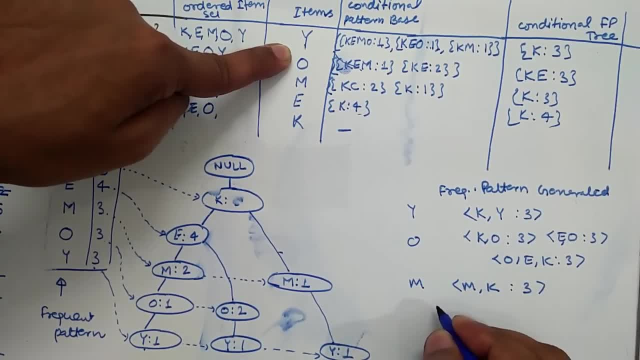 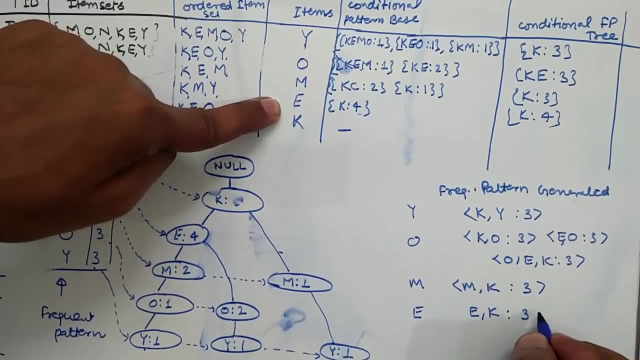 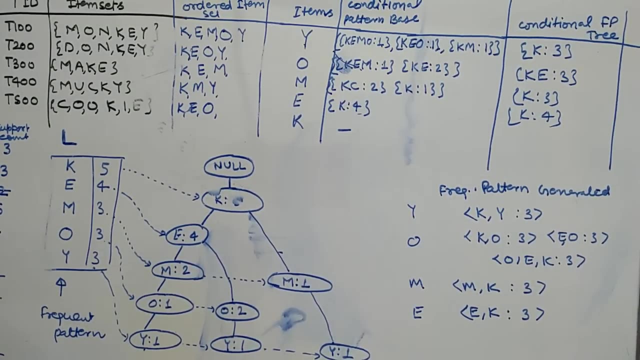 the frequency 3 and from e we generated frequent pattern e, k with frequency 3. okay, so these are the frequent patterns generated by this fp growth algorithm. now the next step is to find out the association rules. so from these patterns we can easily find out the association rules. like for this pattern there are: